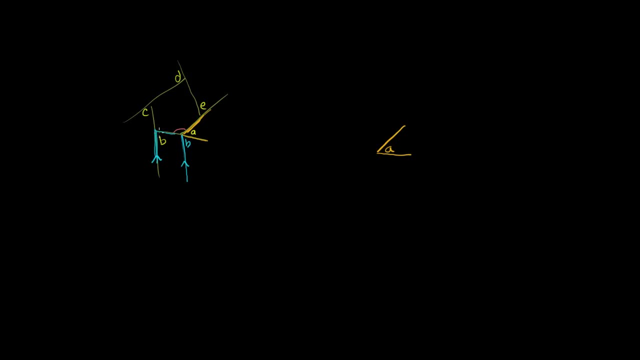 then the measure of this angle right over here would also be B, Because this obviously is a straight line. It would be like a transversal. These are corresponding angles. So if we wanted to draw an adjacent angle- B adjacent to A- 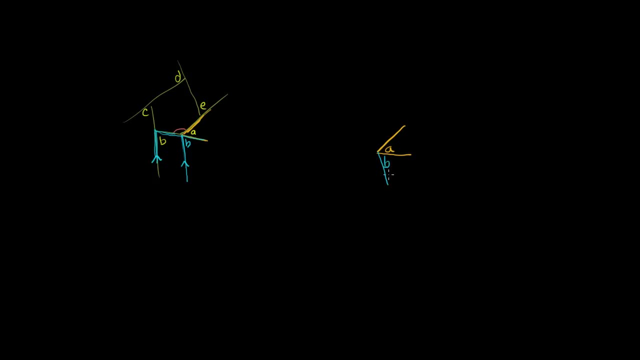 you could do it like that Or whatever angle. this is: its measure is B, And now it's adjacent to A, And now let's draw the same thing for C. We could draw a parallel line. We could draw a parallel line to that right over here. 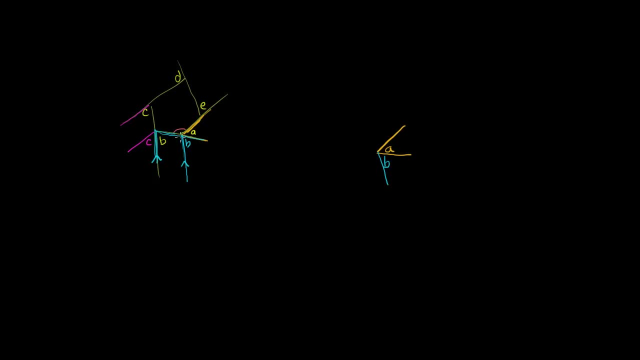 And then this angle would also be C, And if we want it to be adjacent to that, we could draw it right over here. So that angle is C. So C would look something like this, C would look something like that. Then we can move on to D Once again. 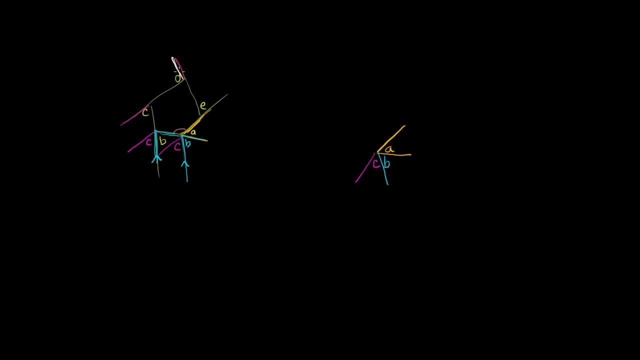 let me do that in a different color. You could do D. D could be right over here, Or you could shift it down over here to look like that, Or you could shift it over here to look like that, If we just kept thinking about parallel. 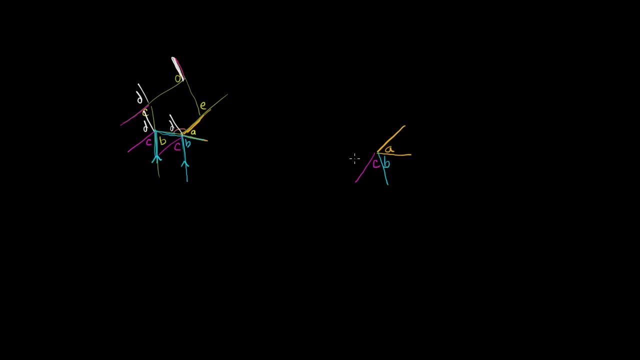 if all of these lines were parallel, if all of these lines were parallel to each other. So let's just draw D like this: So this line, once again, is going to be parallel to that line, And then, finally, you have E. 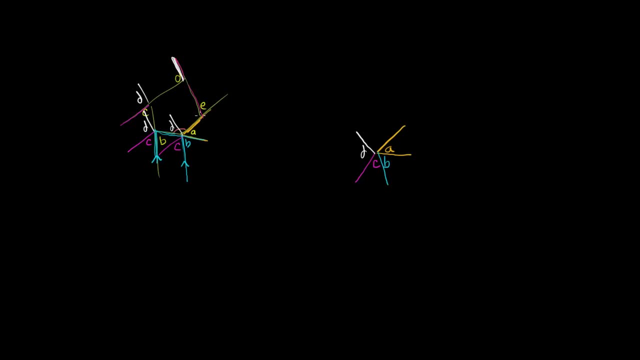 Finally, you have angle E And once again, you could draw a line that is parallel to this right over here, Right over here, And this right over here would be angle E. Or you could draw it right over here, You would draw it right over here. 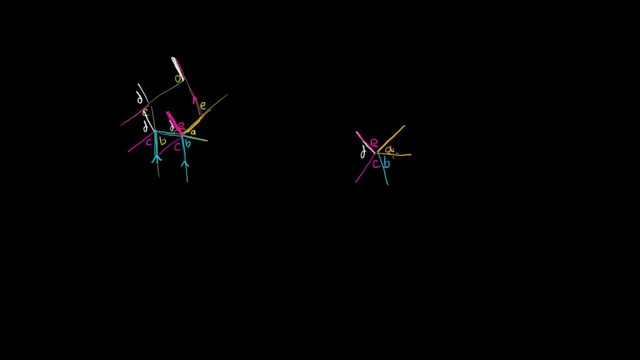 And when you see it drawn this way, it's clear that when you add up the measure, this angle- A, B, C, D and E- you're going all the way around the circle. Either way, you could be going clockwise. 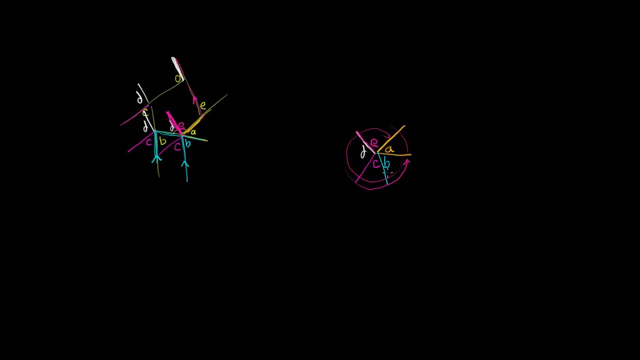 or you could be going counterclockwise, But you're going all the way around the circle, And so the sum of these angles are just going to be so A plus B plus C plus D plus E is just going to be 360 degrees. 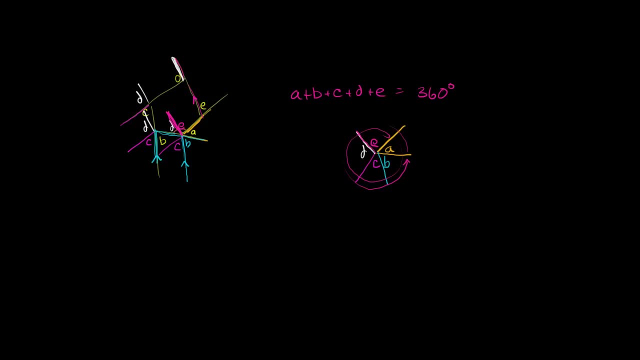 And this will actually work, as I said, for any convex polygon. When I say convex polygon, I mean one that's not dented inwards. So just to be clear what I'm talking about, it would work for any polygon. that is kind of.